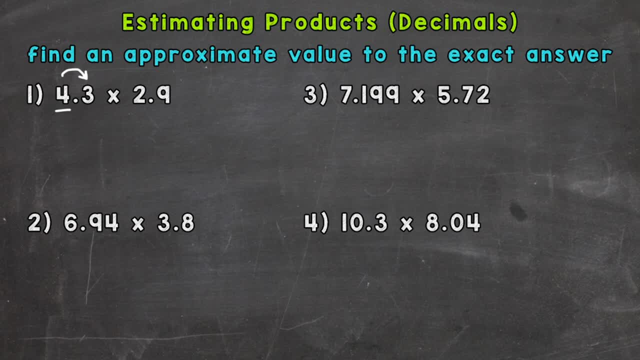 Or is that going to round up to five? Or is that going to round up to five, Or is that going to stay the same at four? Now, four and three tenths is going to be closer to four. That three says stay the same Times. well, two and nine tenths, let's see if this is closer to two or three. 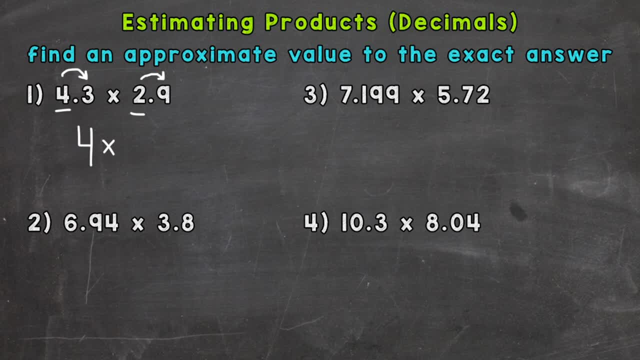 So look next door and that nine tells us that we round up to three, that we are closer to three. So we can do four times three in order to get an estimate here. So our estimate is going to be 12. So we can put four and three. 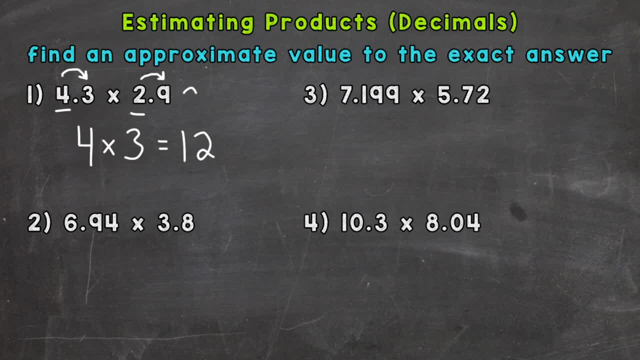 tenths times two and nine tenths is approximately 12.. So this squiggly equal sign means approximately a close value. Now, the exact answer to number one is 12 and forty seven hundredths. So you can see that we had a pretty good estimate there. It was really close to that exact answer. On to number, 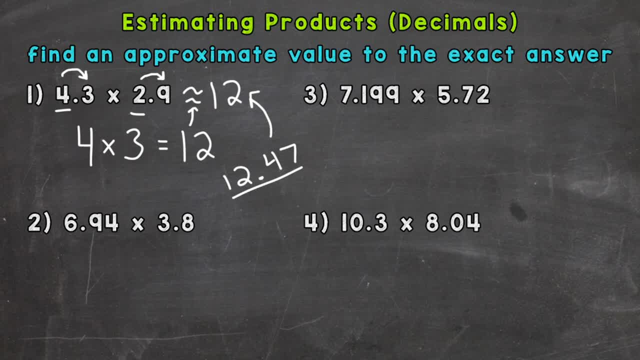 two, where we have six and ninety four hundredths times three and nine tenths is approximately 12.. times 3 and 8 tenths, So again let's round to the nearest whole number. the ones place 6 and 94 hundredths. let's look next door and this is going to round to 7.. 6 and 94 hundredths. 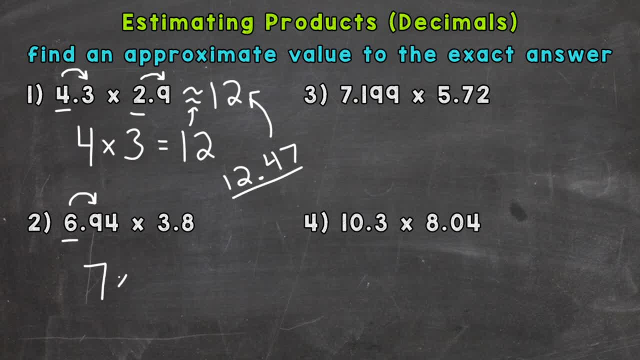 is closer to 7 than it is to 6, times 3 and 8 tenths is going to round to 4.. So we can do: 7 times 4 equals 28,, and that's going to be our estimate. The exact answer to number 2 is 26. 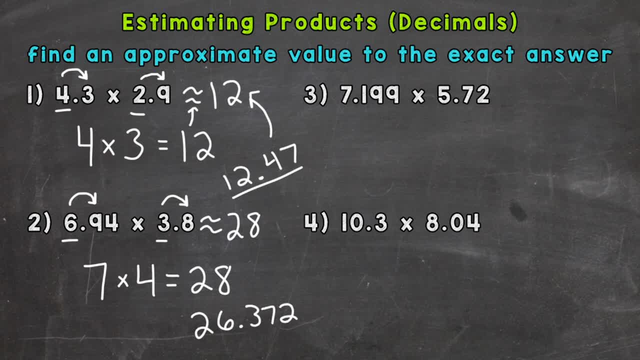 and 372 thousandths. So again pretty close estimate there. That gave us an approximate value to that exact answer. Number 3, we have 7 and 199 thousandths times 5 and 7200.. So let's round 7 and 199 thousandths, rounds to 7, times 5 and 7200 rounds to 6.. 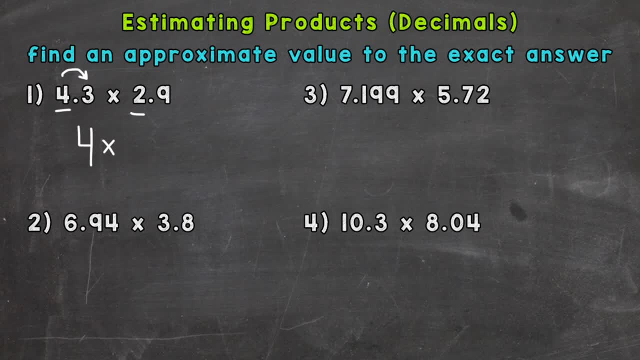 Times. well, two and nine, tenths, Let's see if this is closer to two or three. So look next door and that nine tells us that we round up to three, that we are closer to three, So we can do four times three. 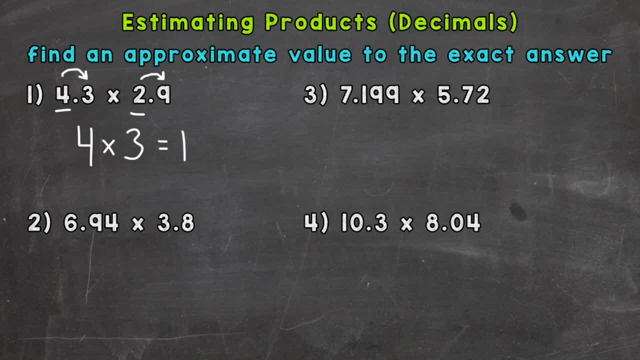 in order to get an estimate here. So our estimate is going to be 12.. So we can put four and three tenths times two and nine tenths is approximately 12.. So this squiggly equal sign means approximately a close value. 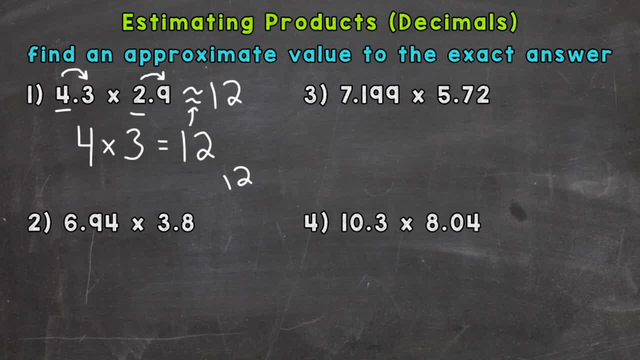 Now, the exact answer to number one is 12 and 47 hundredths, So you can see that we had a pretty good estimate there. It was really close to that exact answer. On to number two, where we have six and nine tenths. 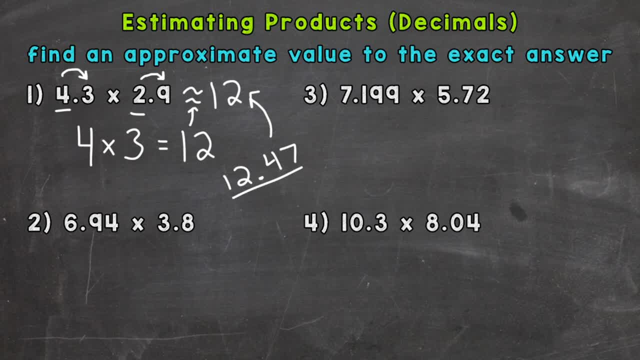 Ninety four hundredths times three and eight tenths. So again let's round to the nearest whole number, the ones place Six and ninety four hundredths. let's look next door and this is going to round to seven. Six and ninety four hundredths is closer to seven. 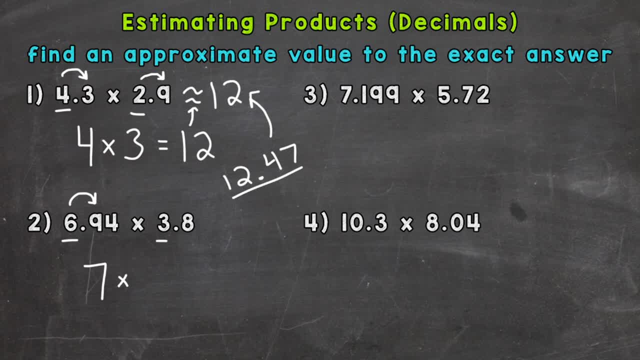 than it is to six Times three and eight tenths is going to round to four, So we can do: seven times four equals 28,, and that's going to be our estimate. The exact answer to number two is 26 and 372 thousandths. 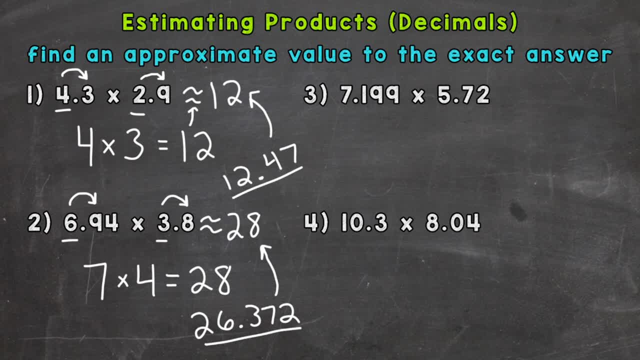 So again pretty close estimate there. That gave us an approximate value to that exact answer. Number three: we have seven and 199 thousandths times five and 72 hundredths. So let's round Seven and 199 thousandths rounds to seven. 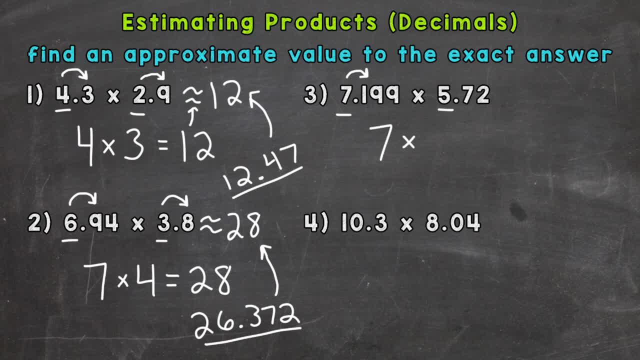 times five and 72 hundredths rounds to six. So seven times six gives us an estimate of 42.. The exact answer to number three is 41 and 343 ten thousandths. So again, we have a pretty close estimate there. And lastly, number four.